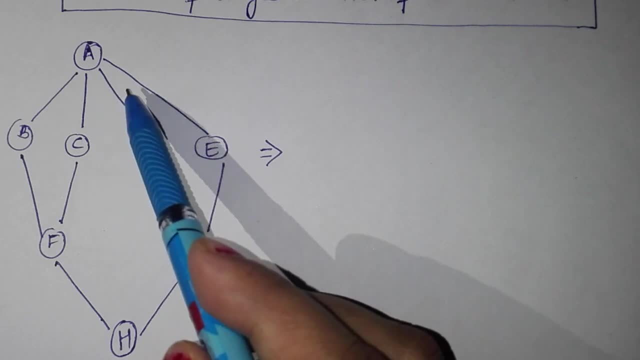 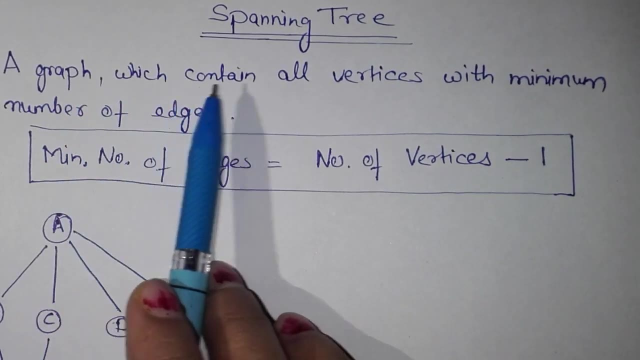 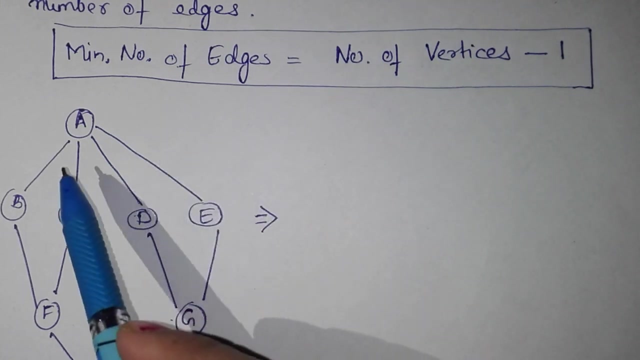 through this edge and A and D connected through this edge, and so on. Ok, friend, now back to Spanning Tree, A graph which contains all vertices with minimum number of edges. It simply means to say, means we need to connect each vertices with minimum number. 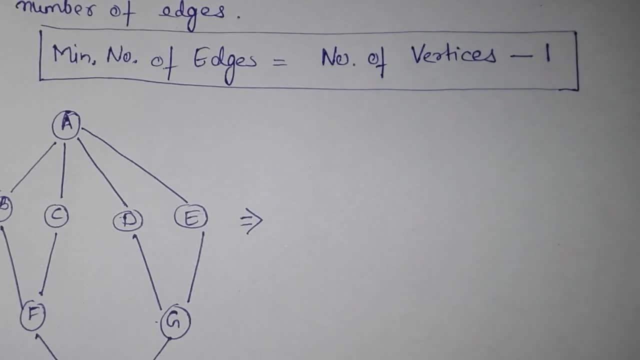 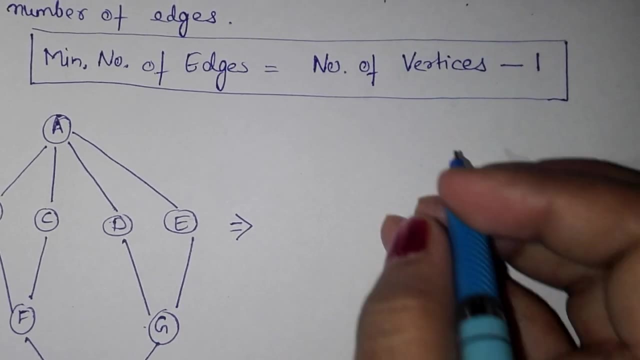 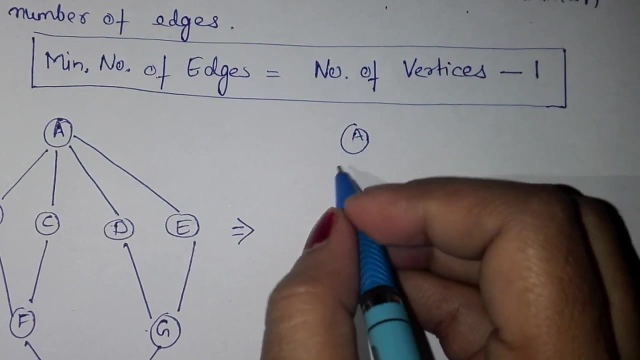 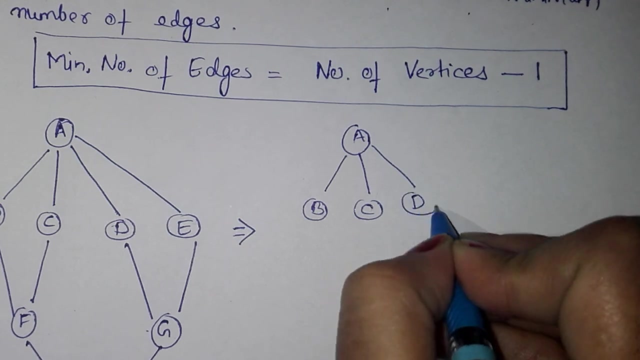 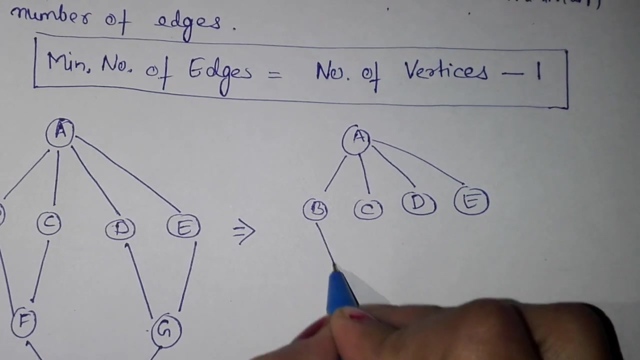 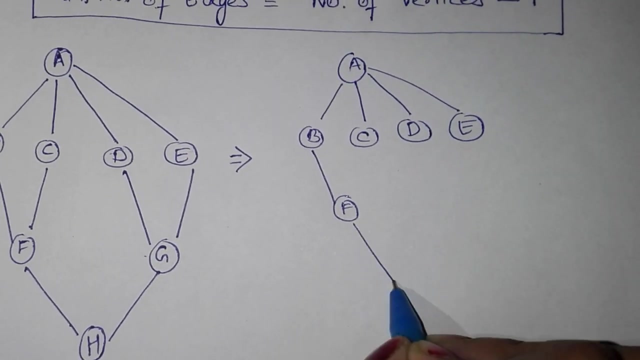 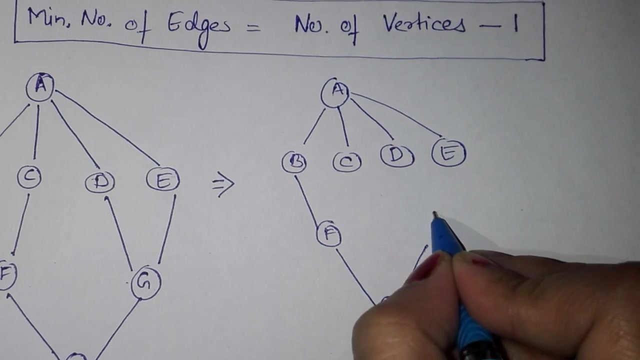 of edges. Ok, So I will show you how can we draw a Spanning Tree for this graph. Suppose this is a graph and we are drawing a Spanning Tree for it. Here we take A, vertices and B and E and B connected with F through this edge, F with edge through this edge, and G. 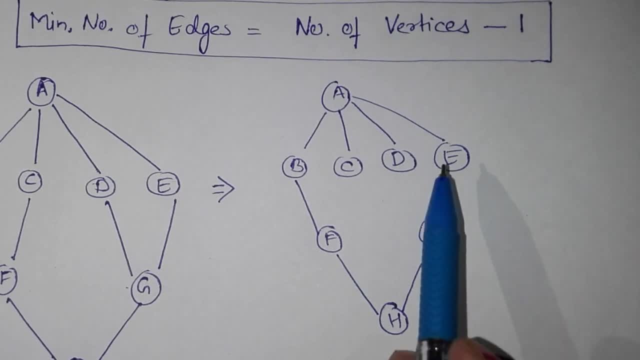 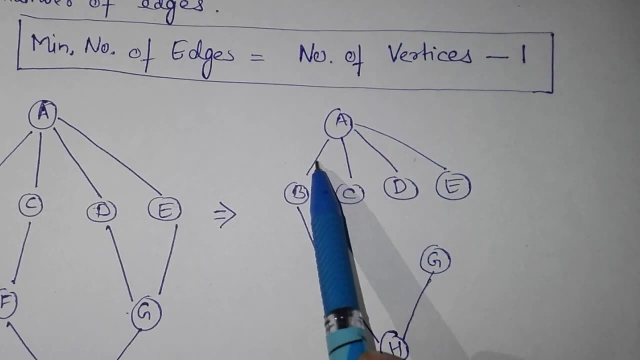 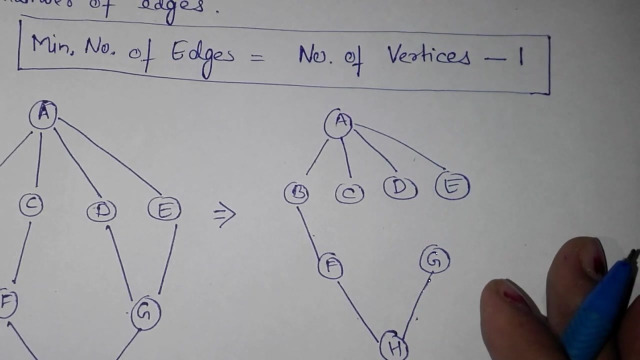 here. So we see here all the vertices are connected. Ok, And number of edges equals to 1,, 2,, 3,, 4,, 5,, 6, 7.. Okay, friends, 7 are the total number of minimum number of edges which are used to draw a spelling tree. 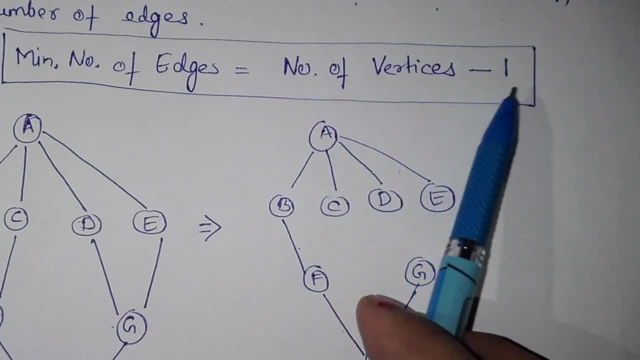 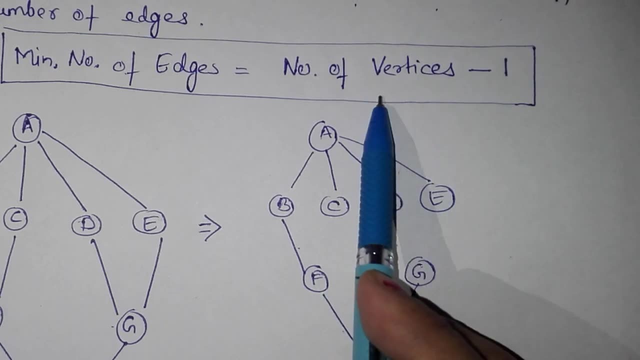 Minimum number of edges equals to number of vertices minus 1.. Here total number of vertices are 8.. 1, 2,, 3,, 4,, 5,, 6,, 7, 8.. So number of vertices is 8.. 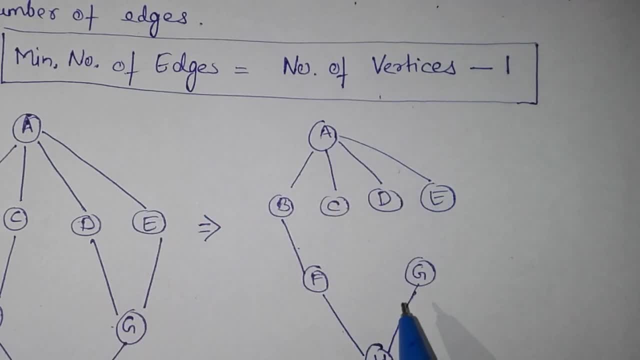 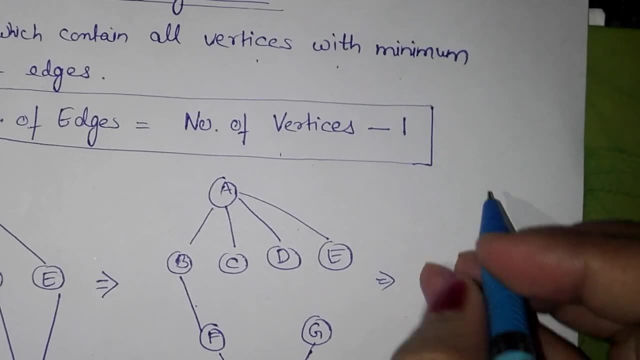 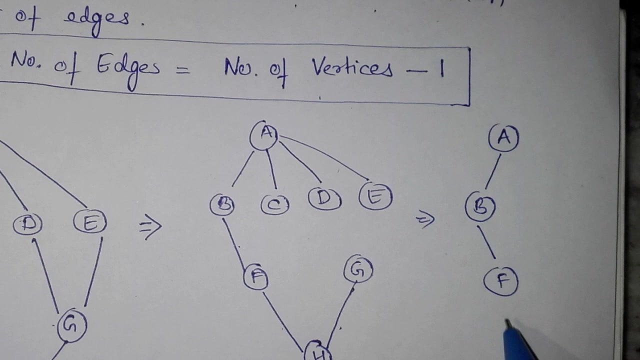 8 minus 1 is 7.. So minimum number of edges are 7.. This is a spelling tree. You can also draw another spelling tree through like this: A, B connect here, F connect it with H, with G. 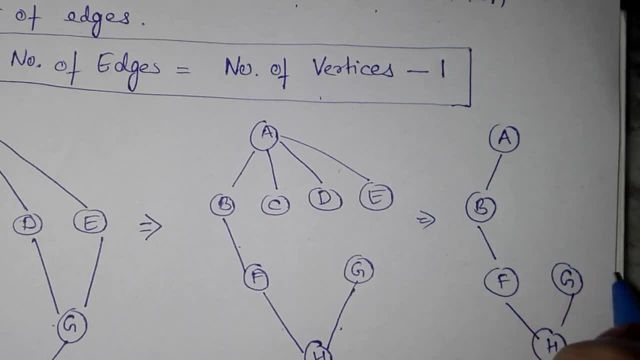 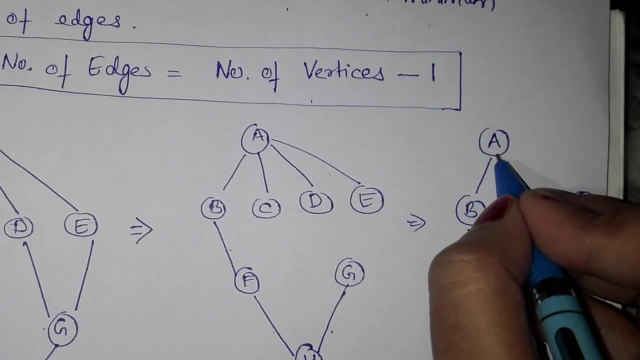 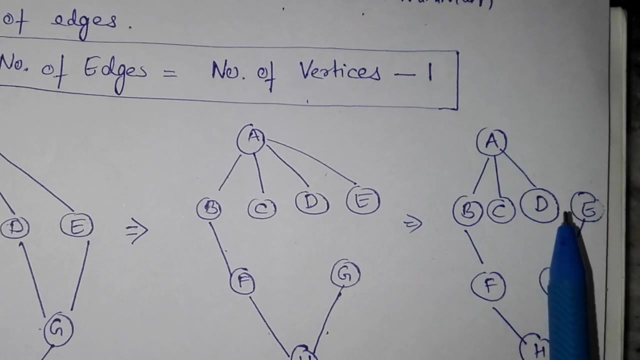 You can connect G with E, Okay. You can connect here A with C, A with D, Okay, friends. So count number of edges: 1, 2,, 3,, 4,, 5,, 6,, 7.. 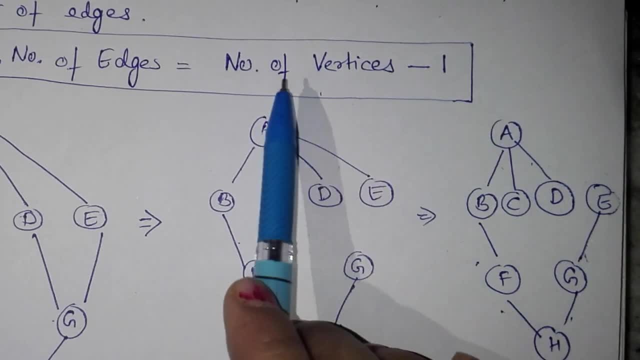 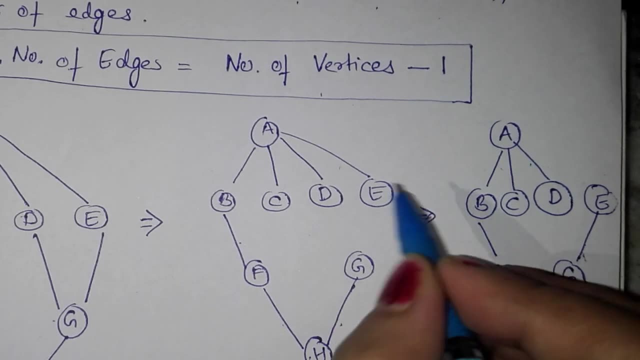 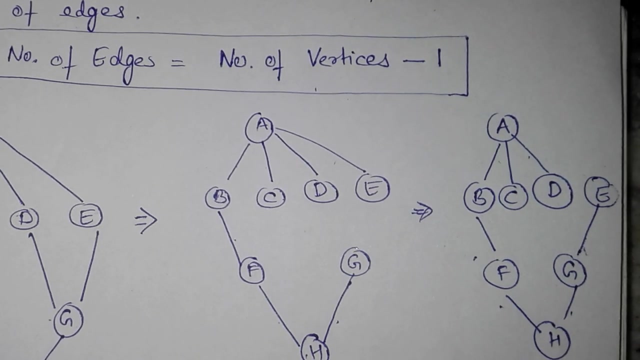 So total number of edges will be 7.. So number of edges equals to number of vertices minus 1.. You can draw any type of spelling tree, But you must remember that number of edges will be always be less than vertices In spelling. 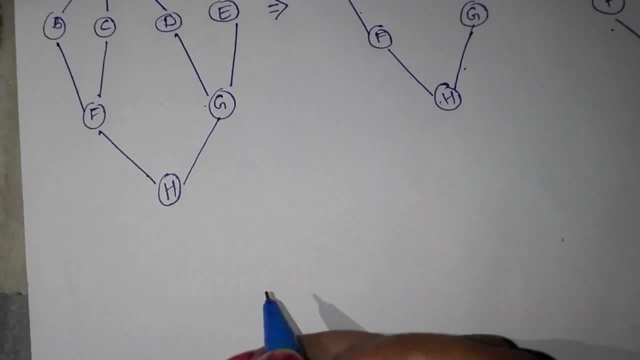 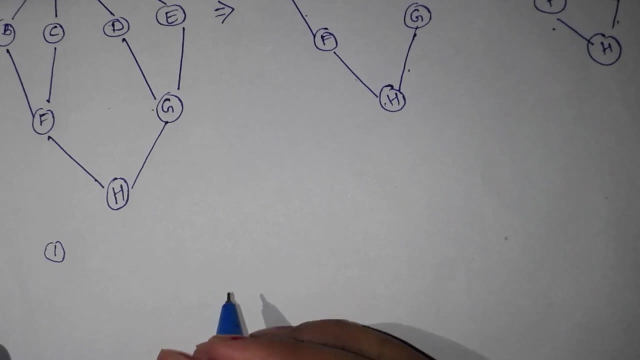 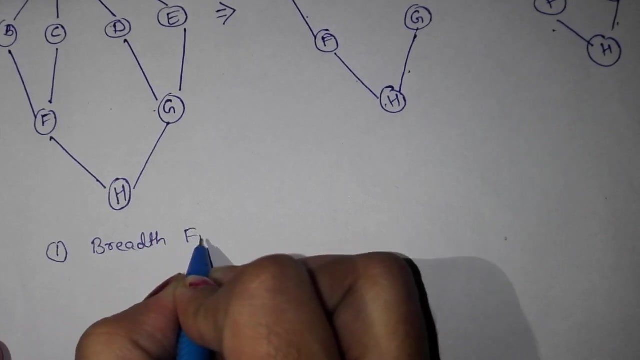 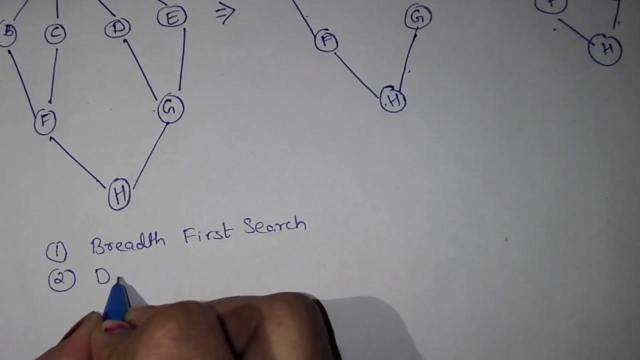 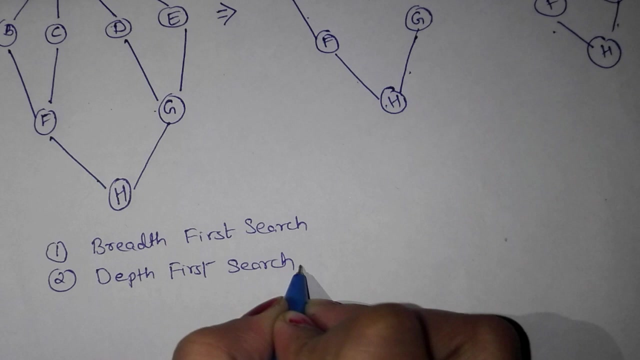 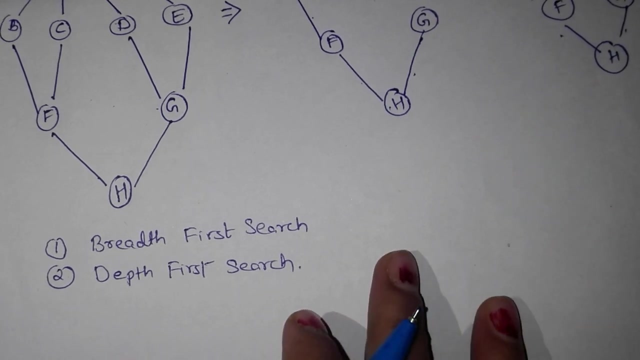 There are two traversing methods. The first one is breadth first search And the second one is depth first search. So these are the two traversing methods which are used in a spelling tree. Okay, So I will explain you one by one. 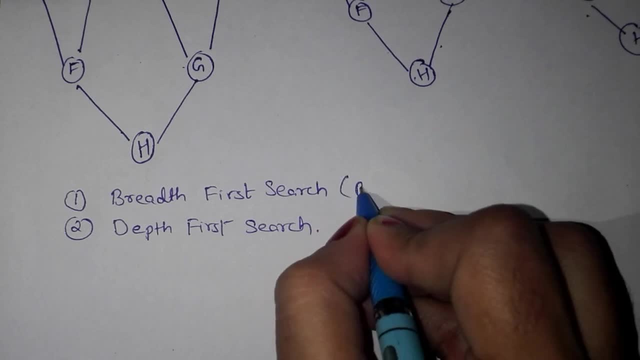 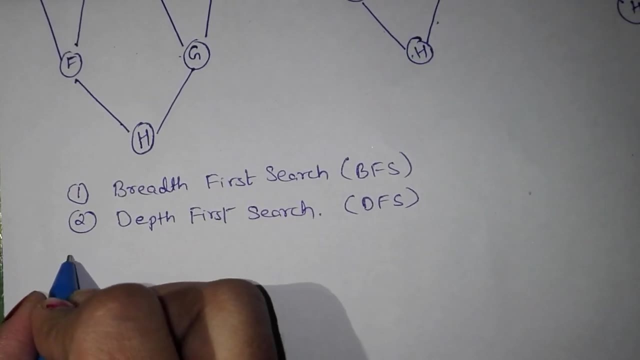 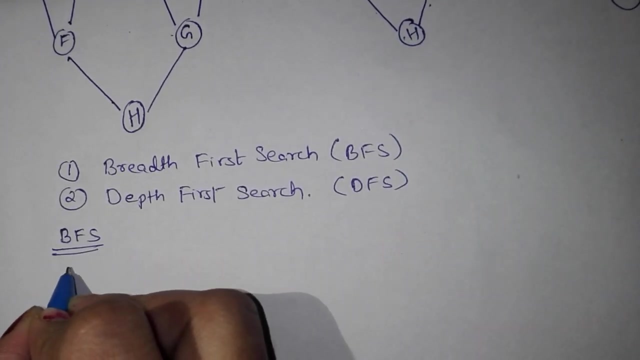 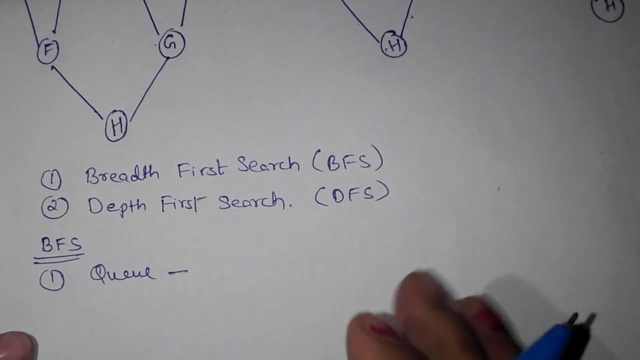 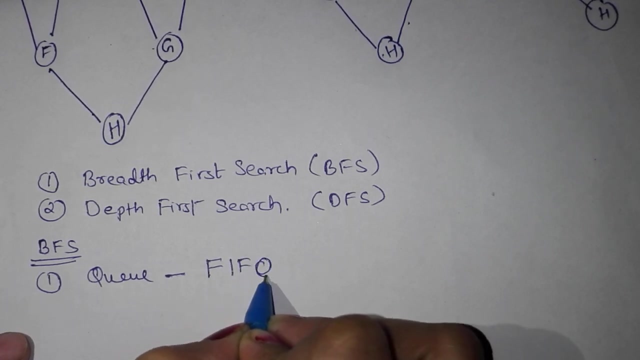 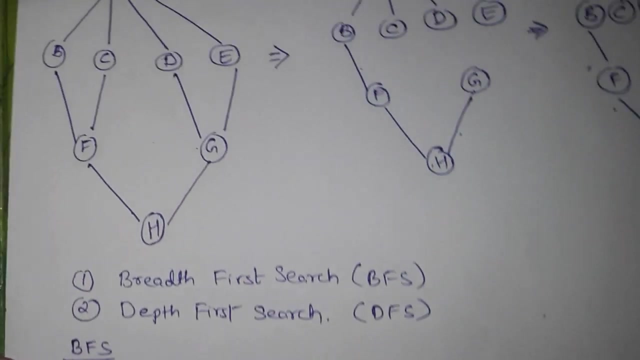 First I will pick breadth first traversing method Here. first point is For breadth first First search traversing method. we use Q. We use Q, As you know, Q is based on FIFO- First in, first out method. Okay, So here I will take the same example. 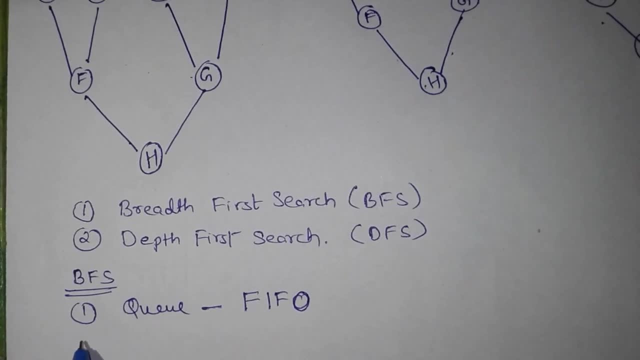 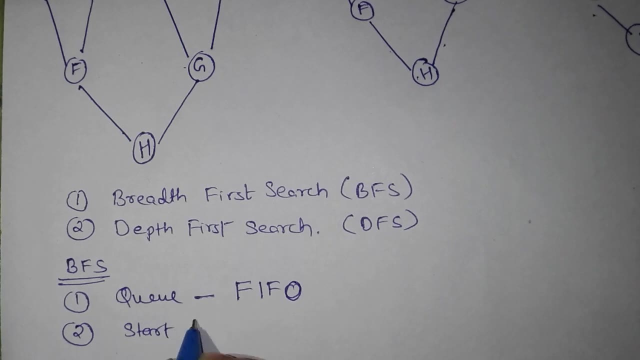 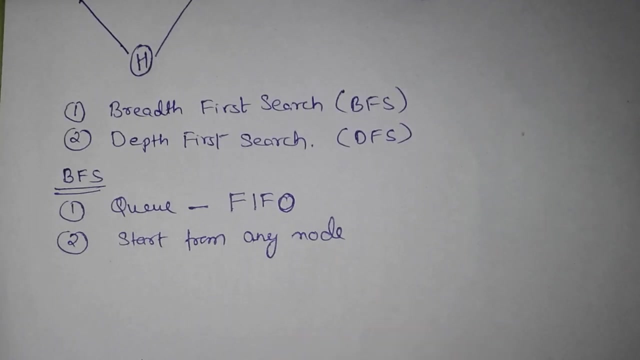 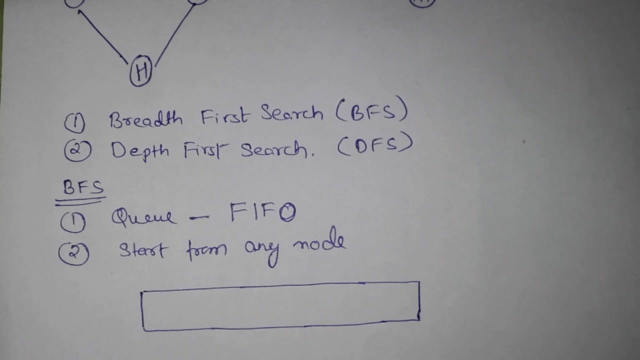 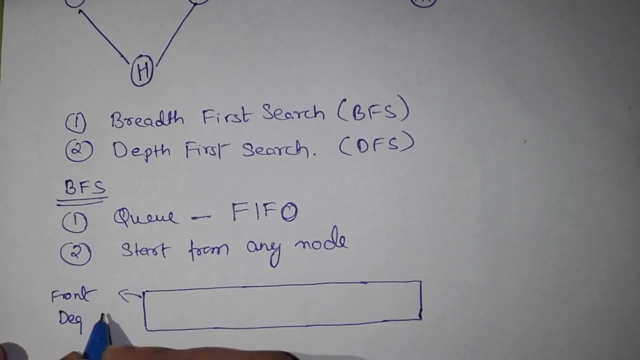 And second point is We can pick any node, Start from any node. Okay, friend, I will draw a Q. This is Q, This is Q. This is front Where we can DQ Means delete the element In Q. 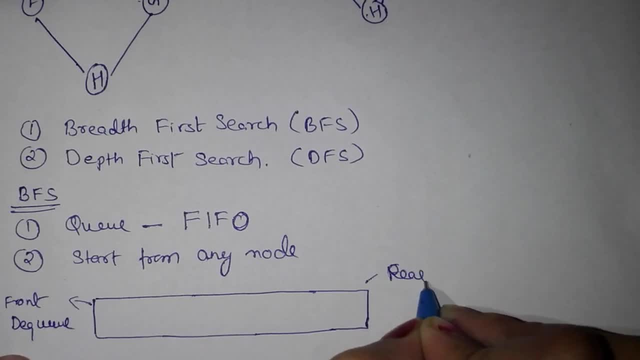 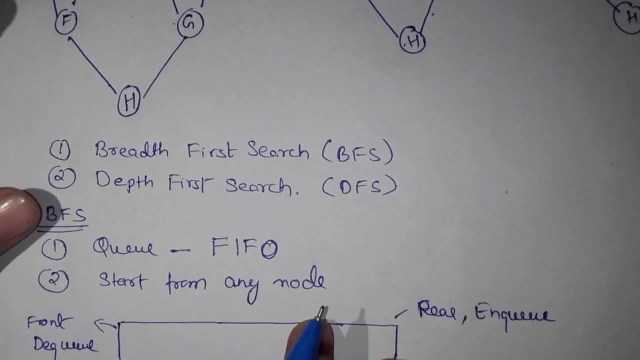 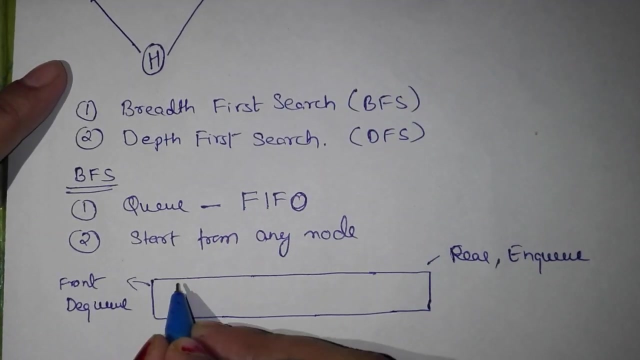 Sorry, this is rear. Here I can add a new element, So NQ. Okay, friend. So Based on Q and start from any node, We pick first node, that is A. Here A is first node. I enter it, This node, in Q. 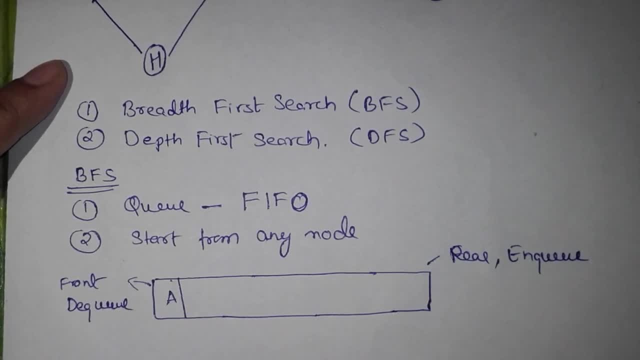 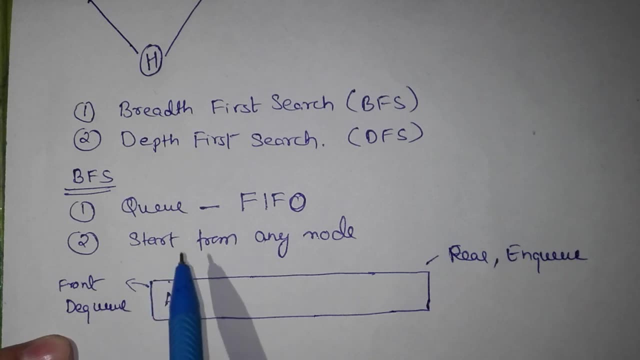 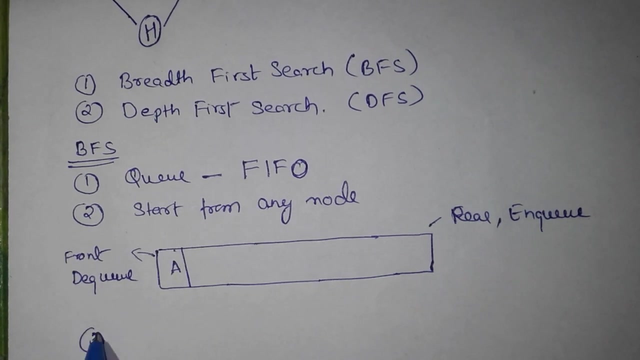 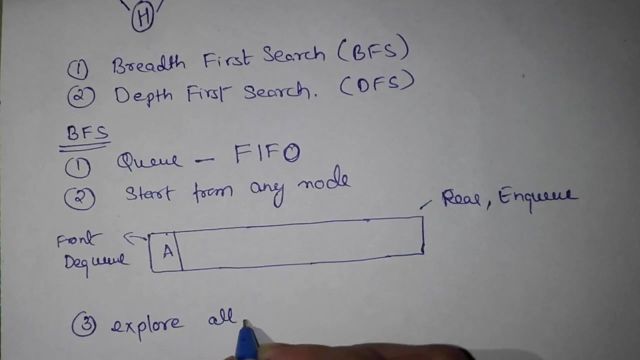 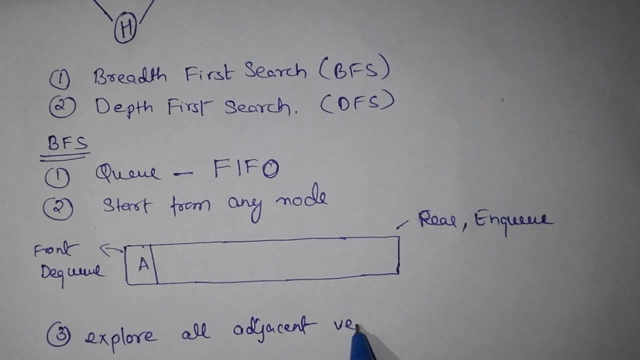 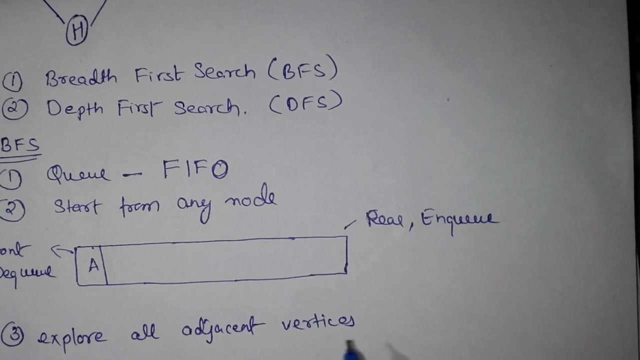 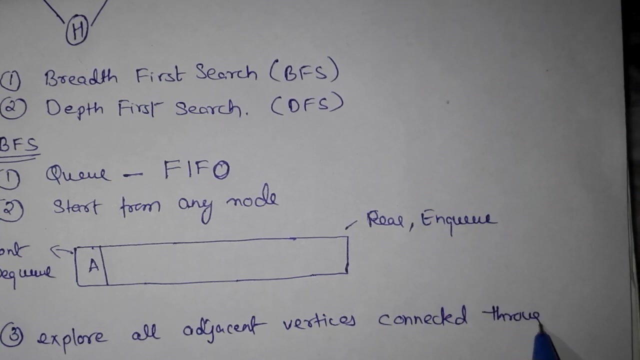 Okay, I enter. A Second point Is completed here And first point also completed here. Number third point is Number. third point is Number. third point is: Explore All adjacent Vertices. Explore all adjacent vertices Connected through: 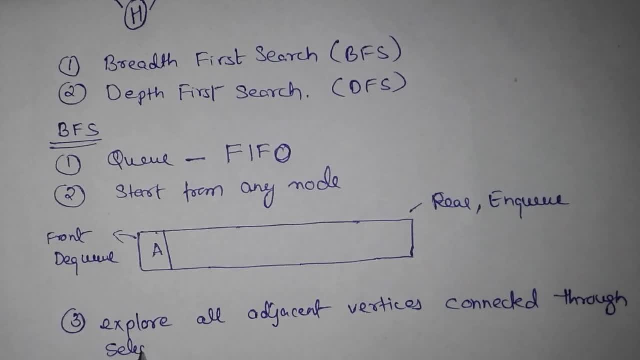 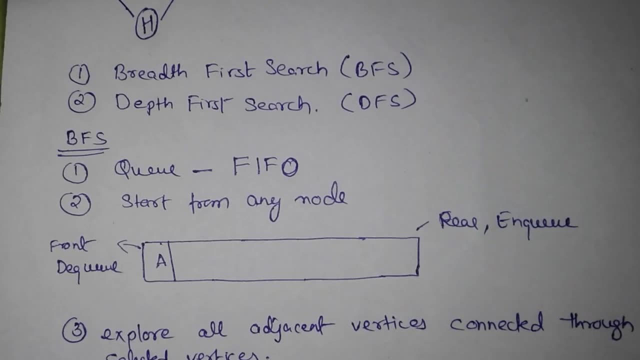 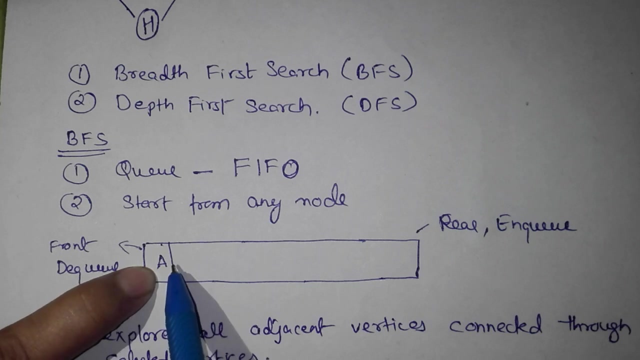 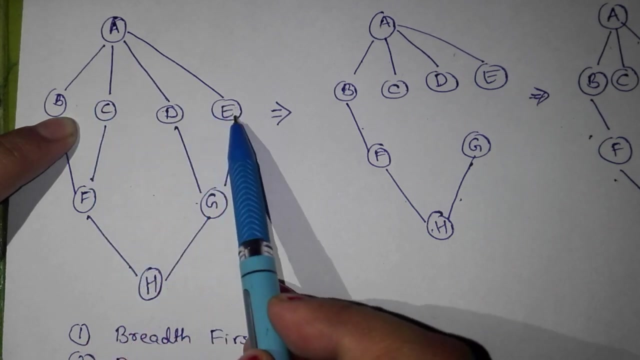 Connected Through Through: Connected Through selected vertices. Okay, friends, So here we selected. first node is A, So explore all the nodes which are connected to A. So here, A is connected with B, C, D and E. So we take: 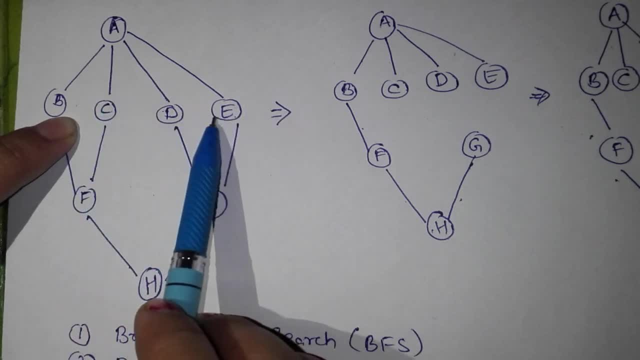 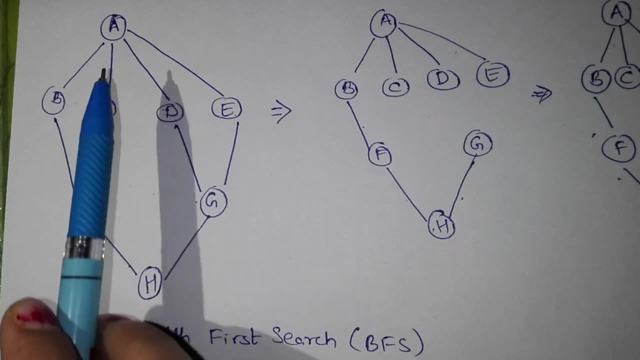 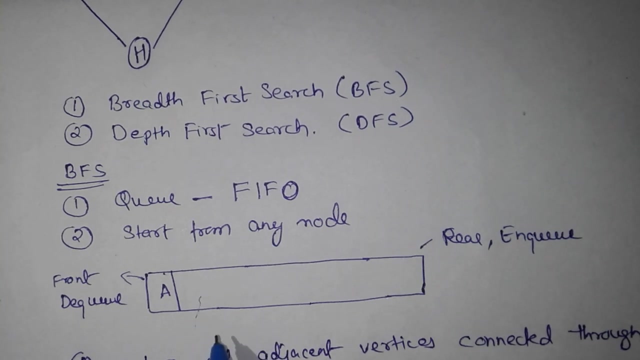 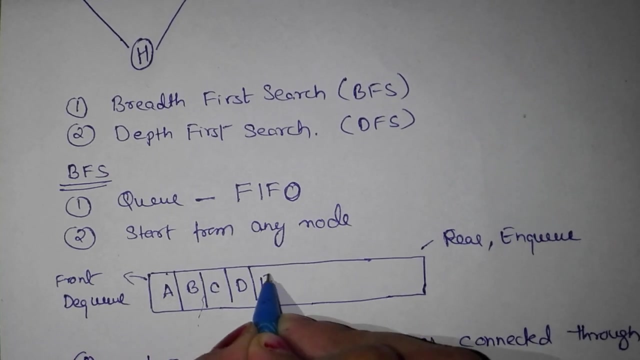 in any sequence: B, C, D, E, or E, D, C, B, whatever your need, you can do anything. So I will select in this sequence B, C, D, E. So A, B, C, D E. Okay, friends, Here our third. 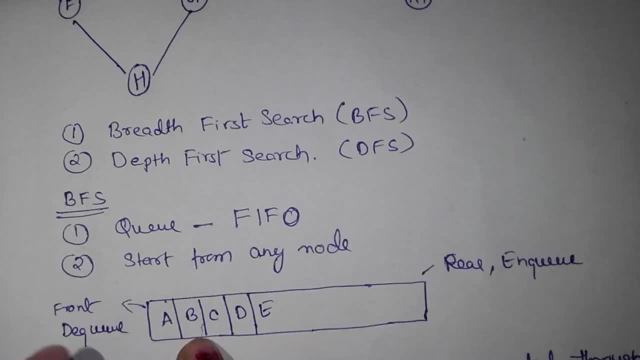 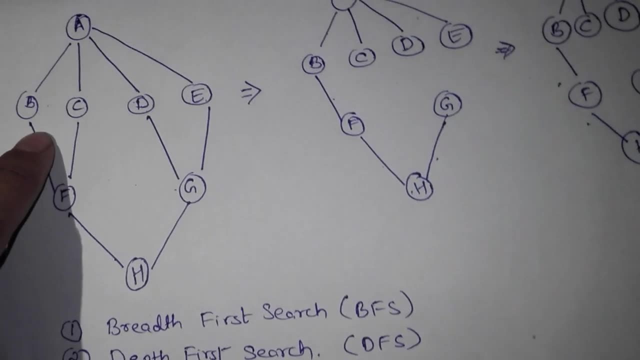 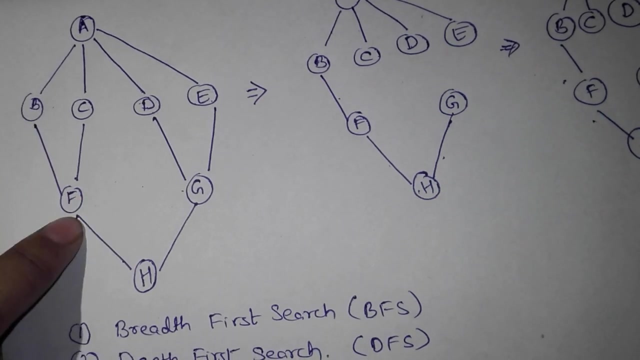 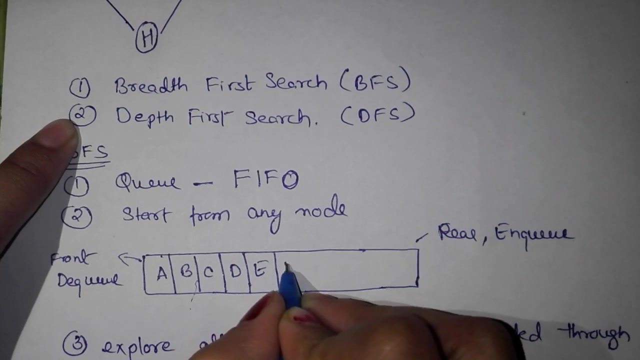 point. So our third point is also completed, Because it is a, Q, So we always take element from front. So B, Take B. How many nodes are connected through B? So F, F is the only node which is connected through B. Okay, friends, So we write here F, Now take next element, C. 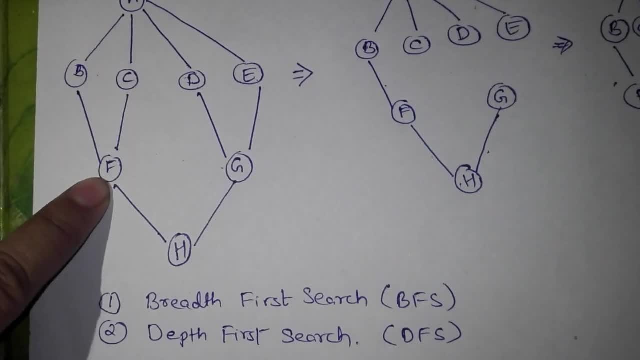 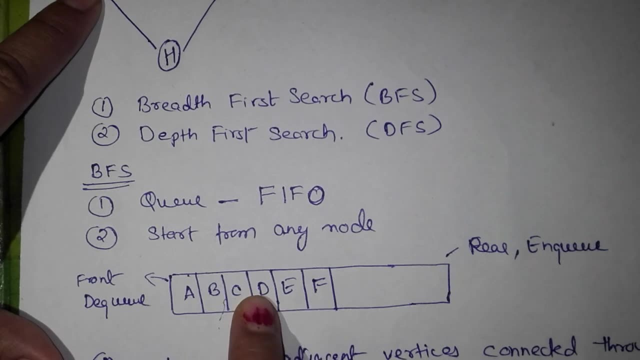 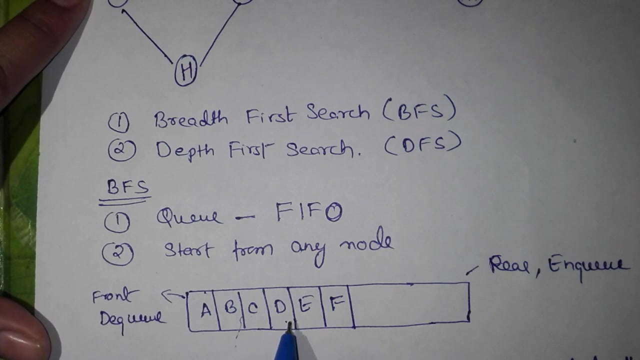 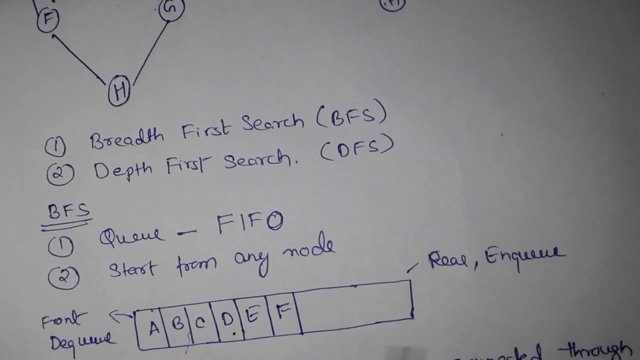 C is connected with again F, F. we already write here Written here This one. Now take D. We always select element from front, So take D Here D is this one. D is connected with G, So we write here G. Take E Here D is connected with G, So we write here G Take. 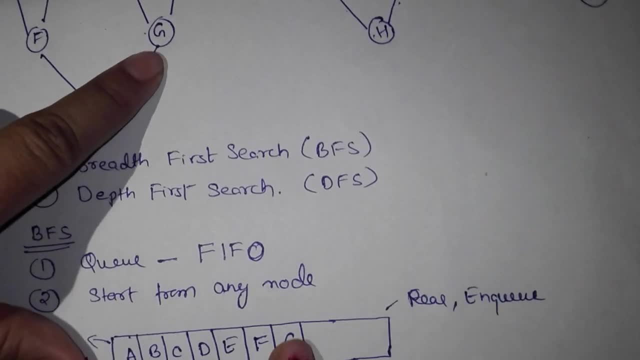 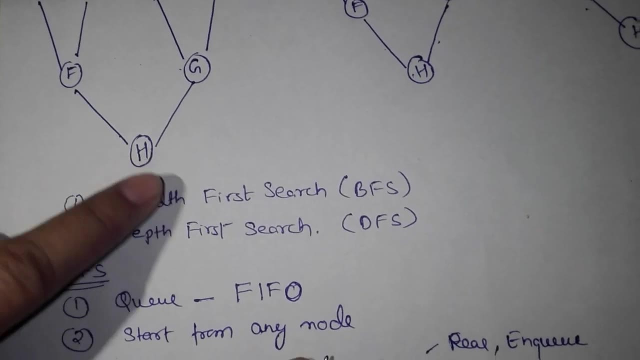 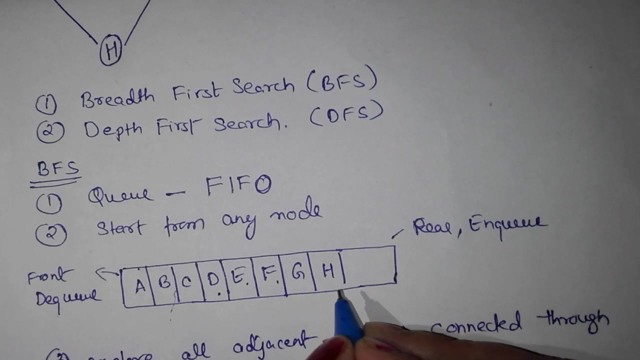 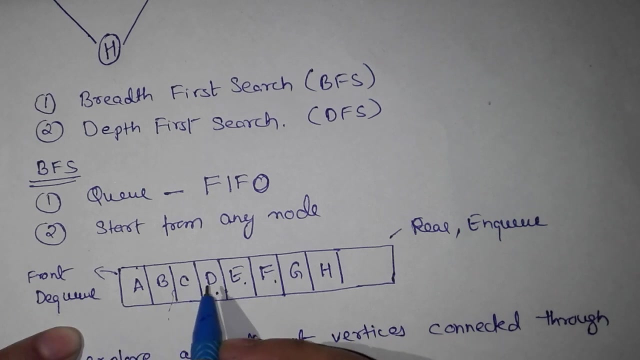 E. E is also connected with G, Which already written here. Then next is F. Take F, and F is connected with H. So here we traversed all the node with minimum number of edges. So the traversing sequence is A, B, C, D, E, F, G, H. Okay, friends, This is breadth. 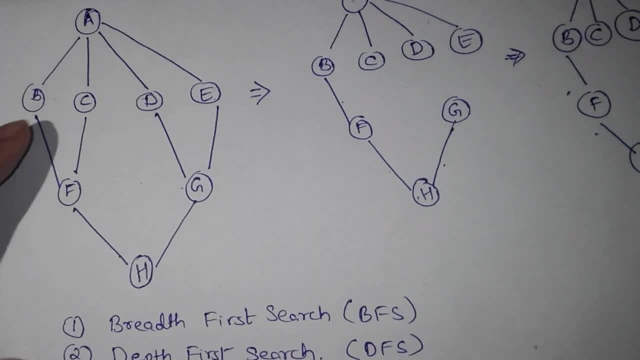 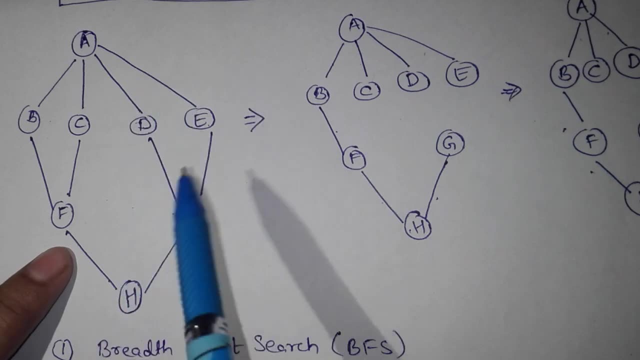 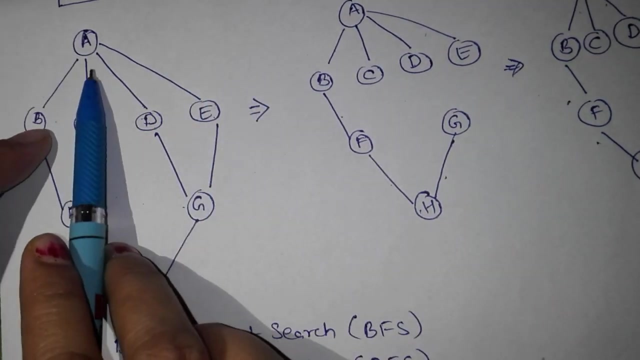 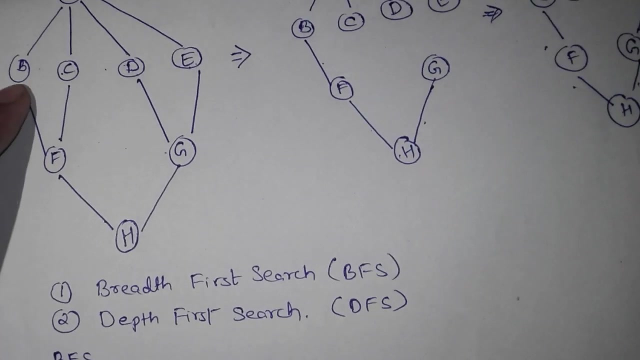 of element. So what kind ofぎN orกn or sixth dimensional growth? So third component is determined as first search. First we select any node. You can select B, either B, either F, either H, any node and then select all the adjacent nodes connected through that node. 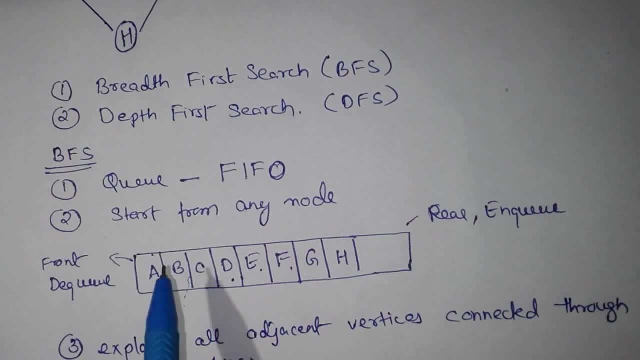 So it's directed to B, C, D, E. I write all the nodes in the Q Here: B, C, D, E. Now select that node and find B. So what is it? So it's written here now. So we write here: B, C, D. 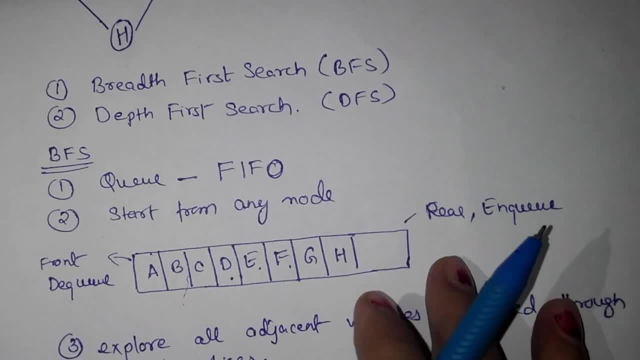 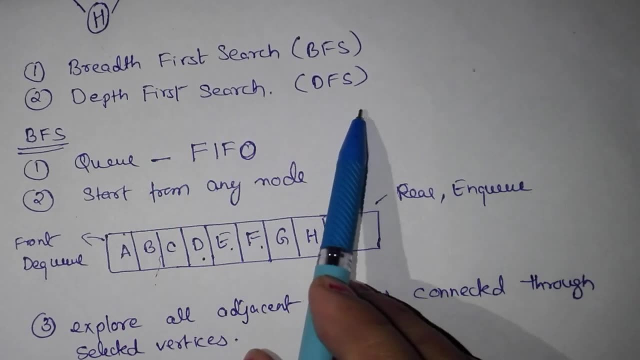 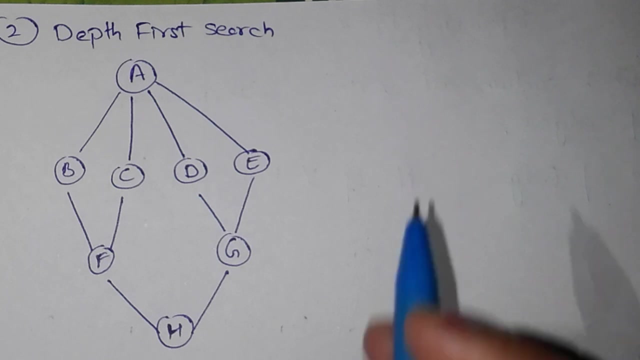 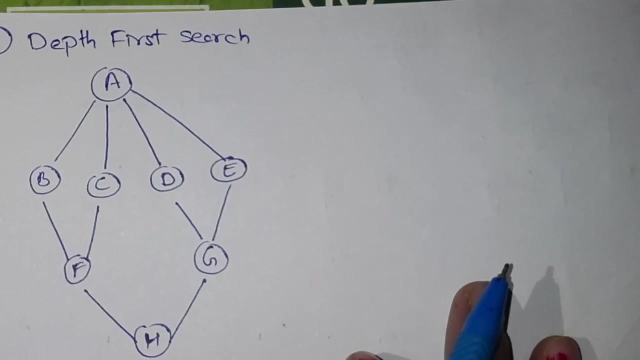 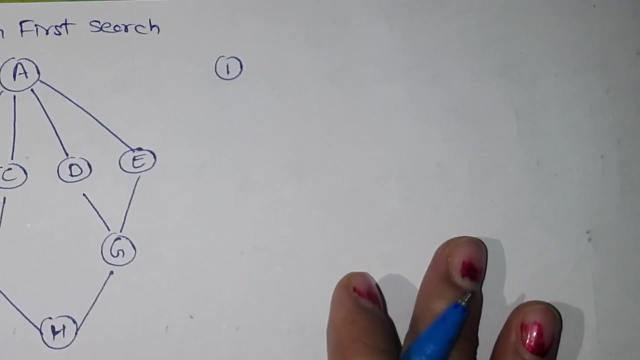 find their adjacent node. okay. so this is how we do: breadth first searching- okay, now move towards depth first search. now we see depth first search. here we take same graph. now there are few points in depth first search is. first point is this: traversing is based on stack. we use stack for the traverse of spanning. 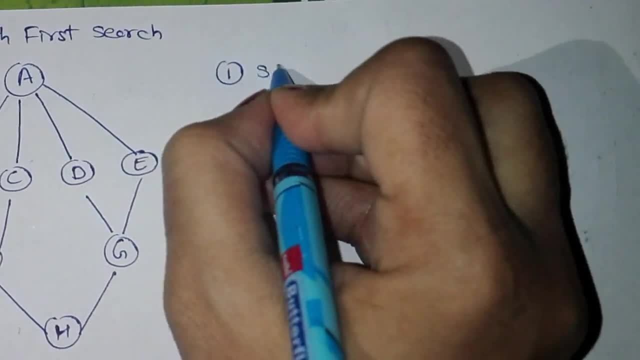 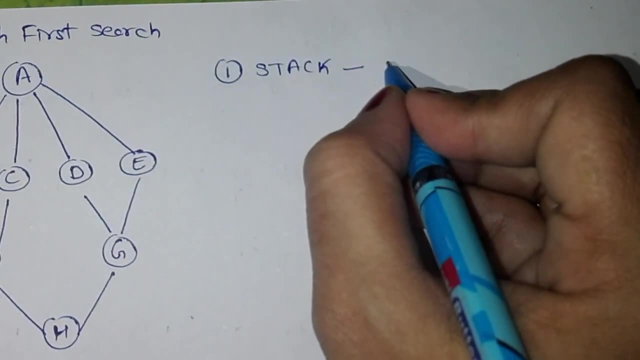 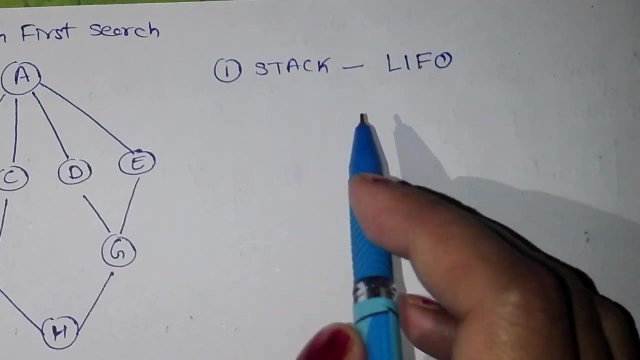 tree in depth first search. so we use stack. as you know, stack is based on leafo, last in, first out. we use push and pop technique in stack. second point: we take süttu, this, two points in last var and the three points other side. we are. 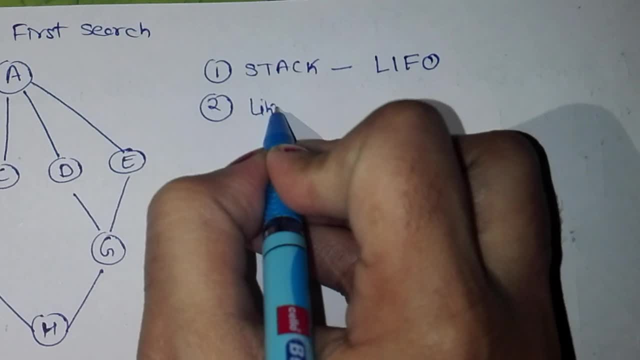 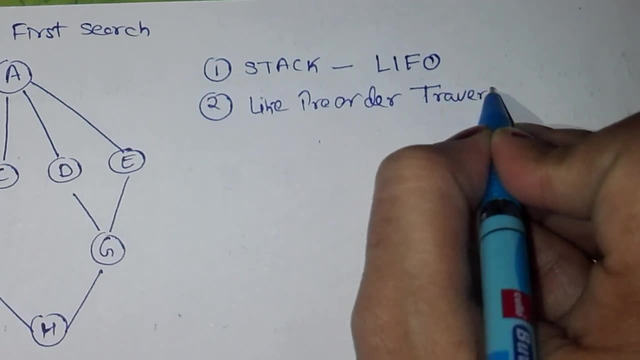 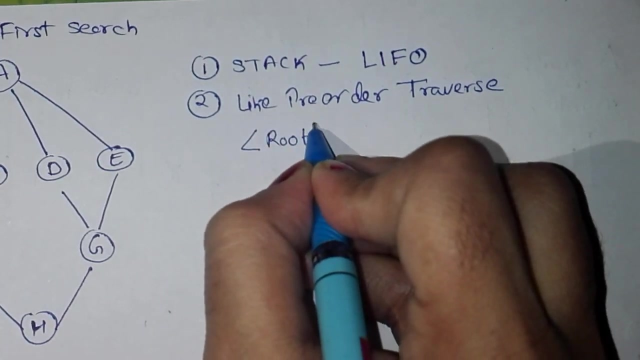 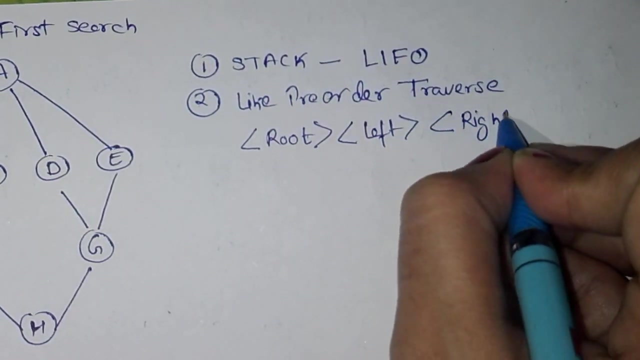 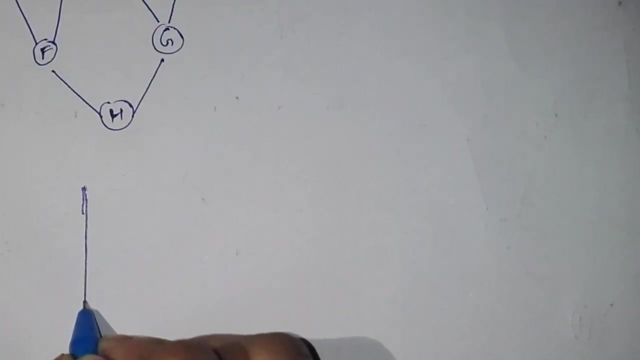 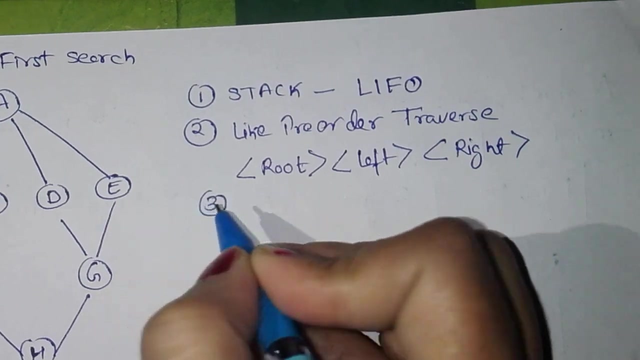 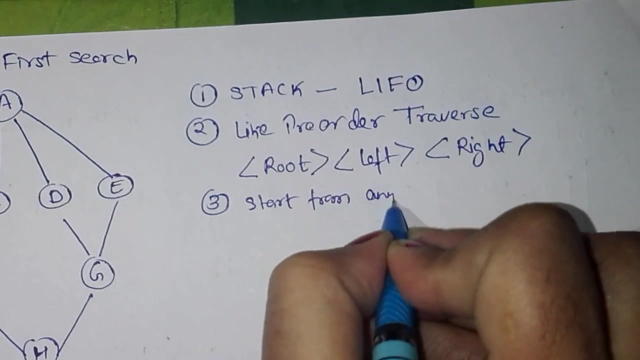 using b and81. okay, si, So start traversing this. We draw a stack. Okay, This is an stack Stack. Third point is: we can start from any vertex. Start from any vertex. So here I will start from A. 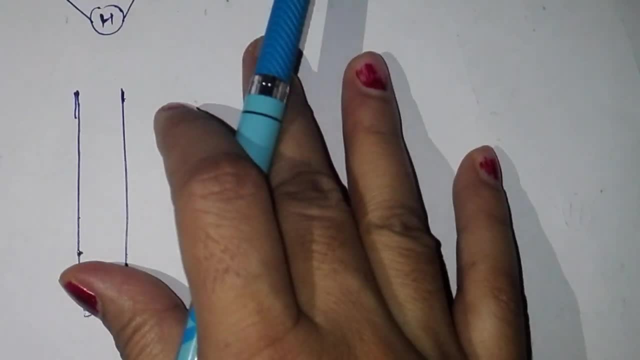 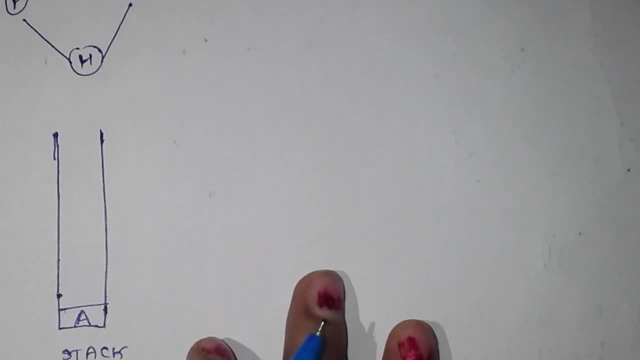 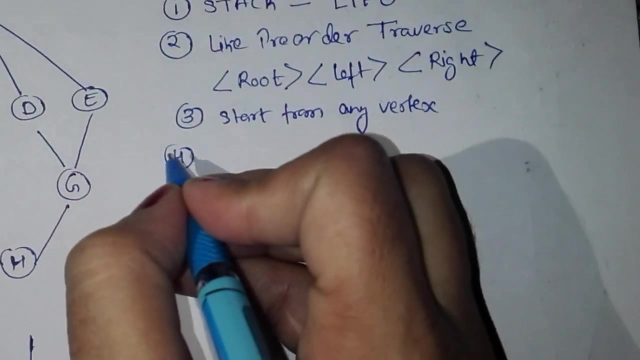 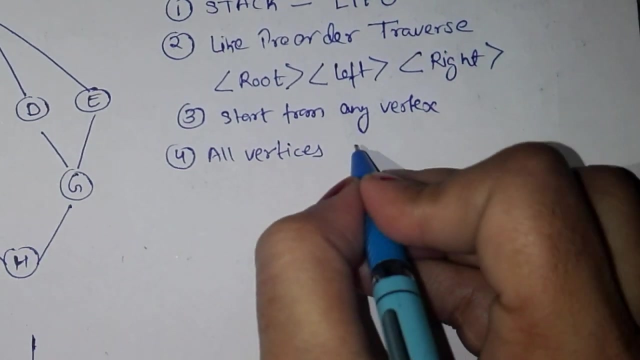 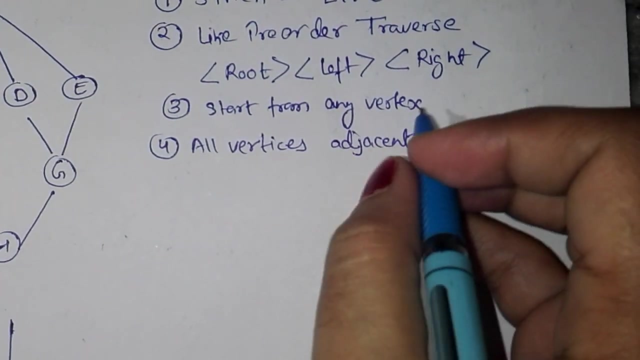 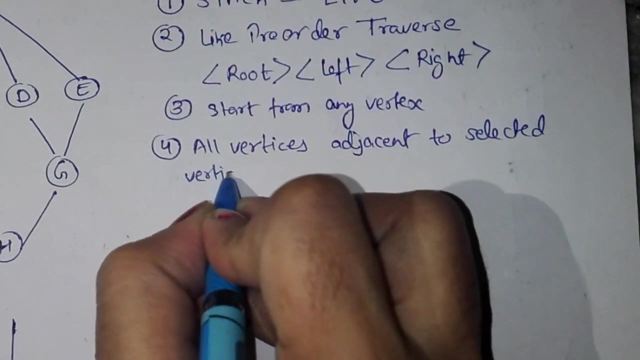 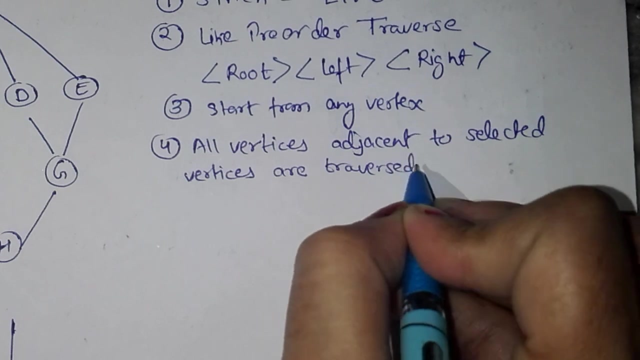 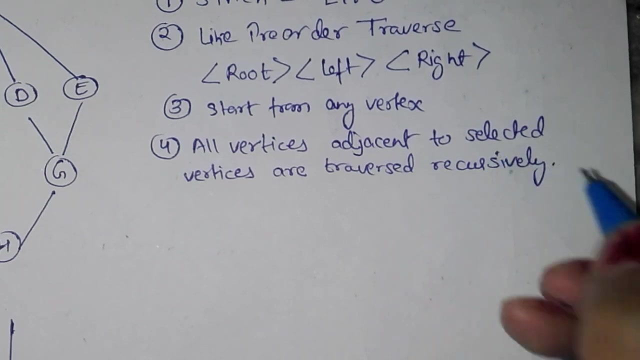 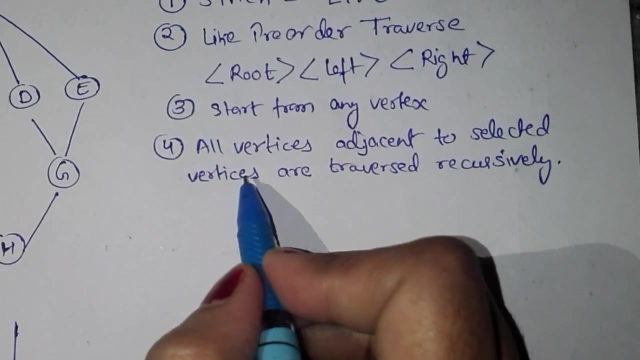 Here I will start from A. So we put here A. Now which node I need to traverse first? So number fourth point is: all vertices adjacent to selected vertices are traversed recursively. All vertices adjacent to selected vertices. Here A is selected. 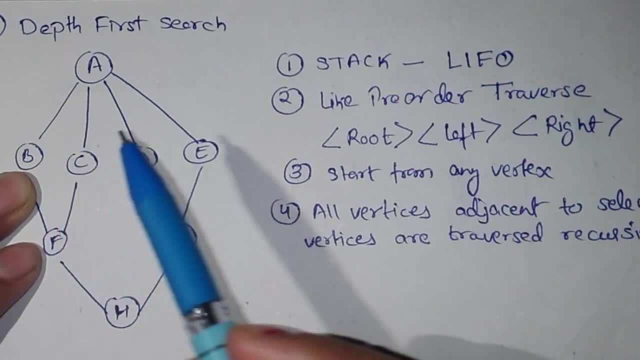 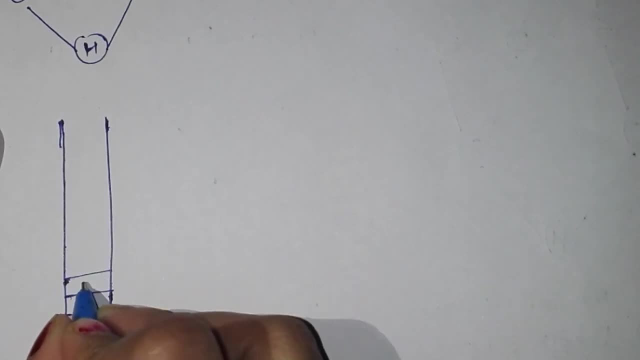 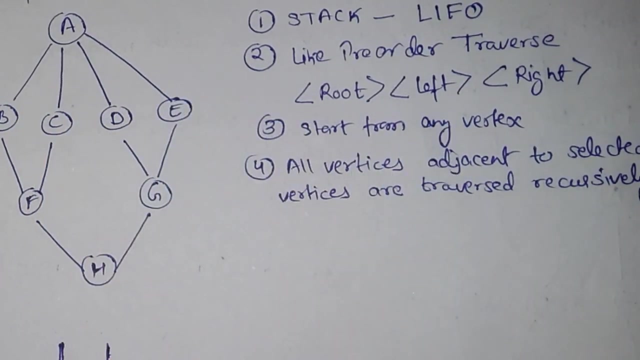 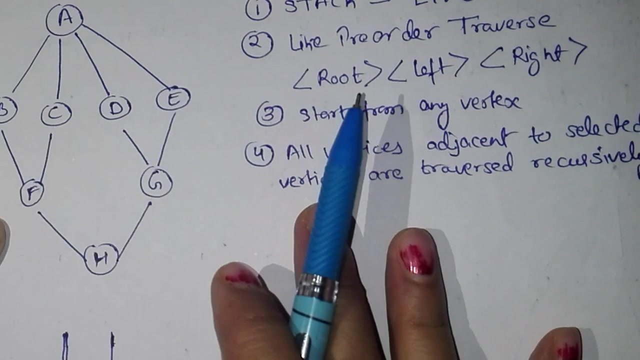 vertices Adjacent to vertices A is B, So we traverse B. So in stack we put B. We don't need to traverse all the vertices at a time, We just put it in a stack. B and now selected vertices is B. We just find next vertices which is connected to B. So here 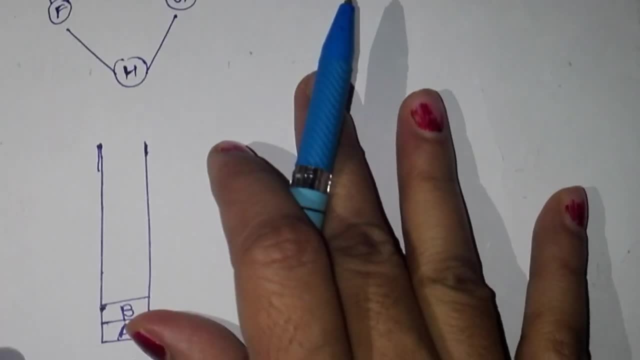 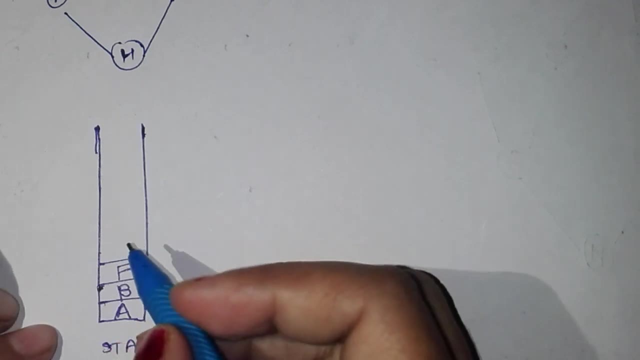 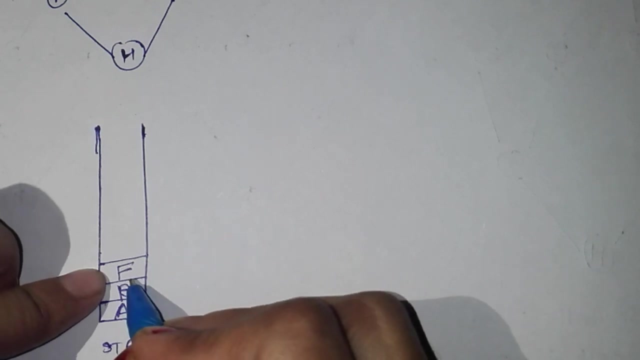 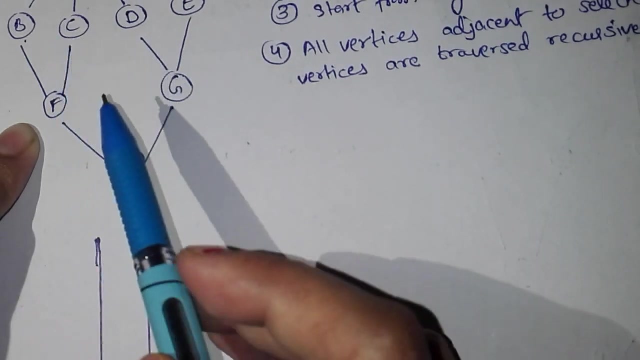 B is connected with F, So we put F here. As it is a stack, we always use top element. Now we find next vertices: which is connected to F, So F is connected to H. F is connected to C. Okay, friend, So here we take C. You. 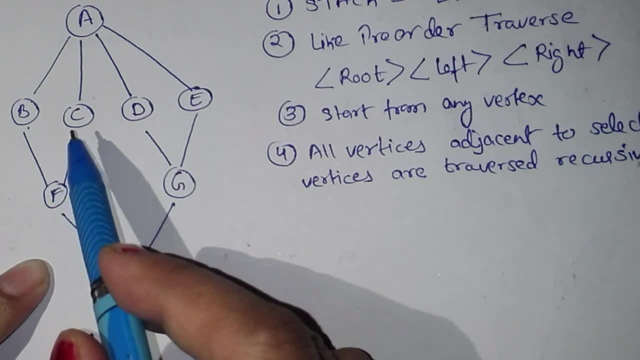 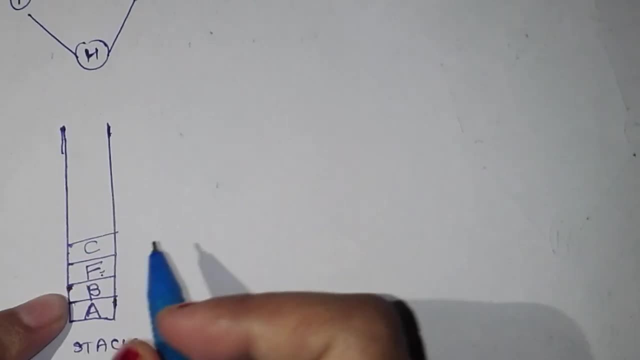 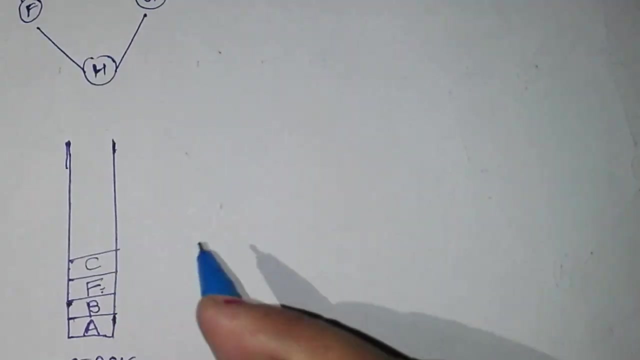 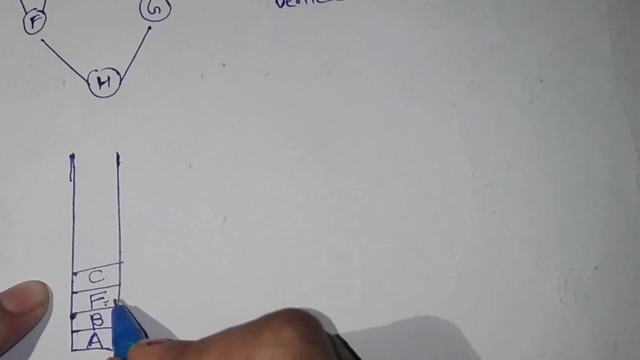 can also take H. Okay, So F is connected with C. Now top element is C. Here C is connected again with A. A already traversed. This one is A. So we see the next top element, F, and F is now connected with H. Okay, So here. 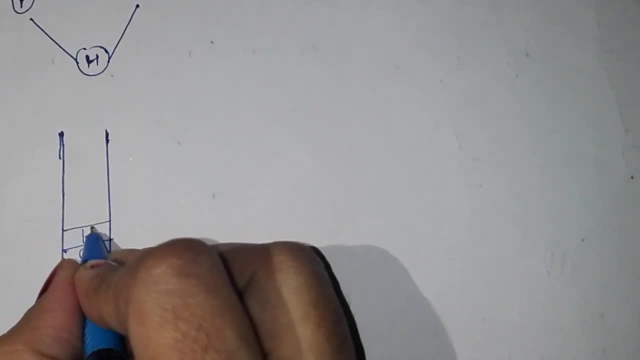 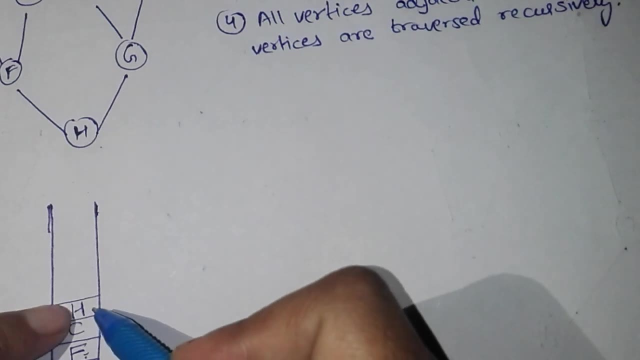 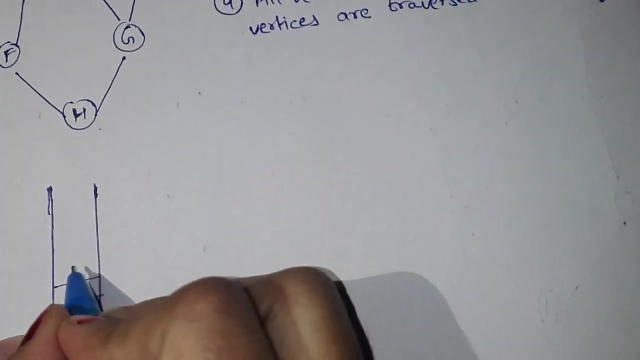 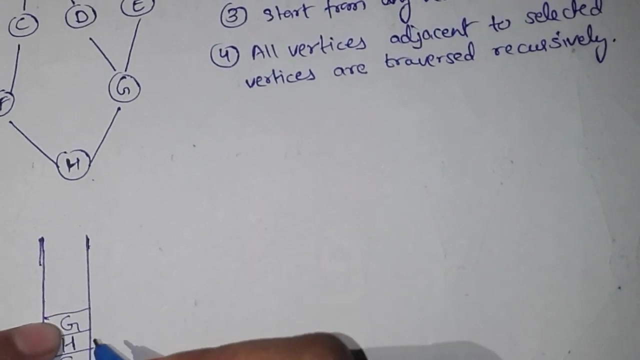 we put H in stack. Okay, Now C. Now C: Which node is connected with the top element of stack? That is H? G is connected with H. So we put here G in stack. Okay, friend. Now top element is G. Which node? 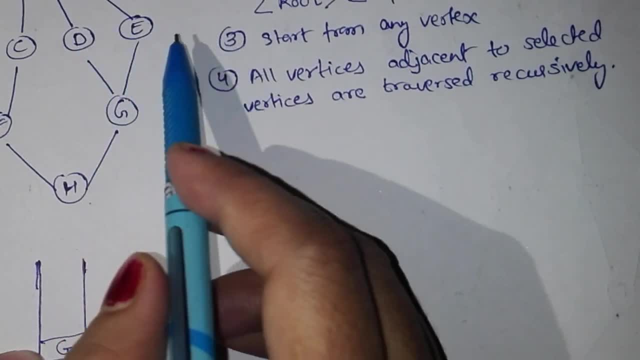 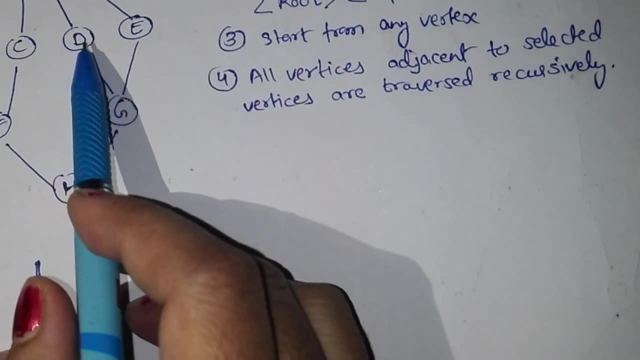 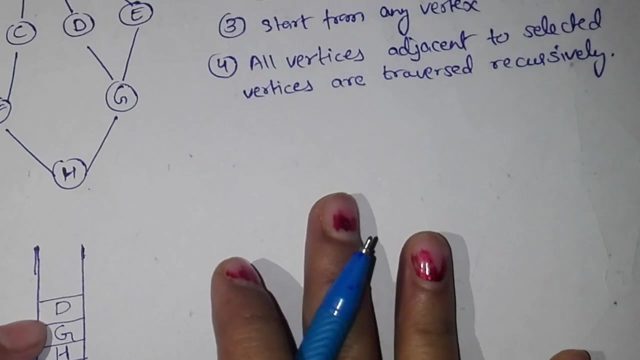 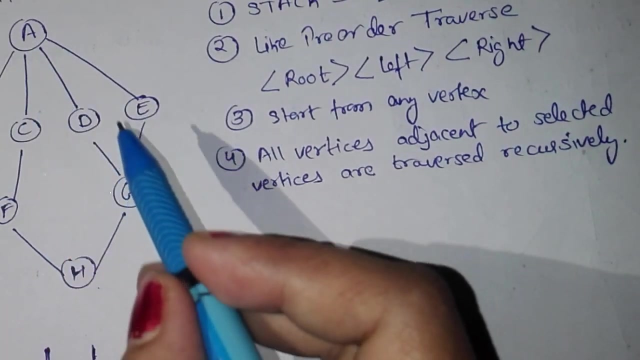 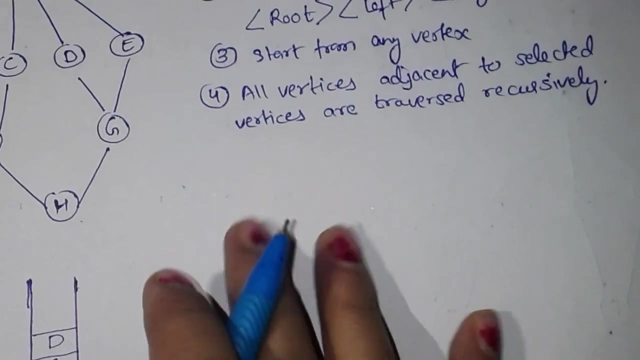 is connected with G. We see D and E, So we can take anyone, either D or E, So I will take D. Okay, Now top element is D, Which node is connected with D. D is connected with A, which is already traversed, So we back to one step. Next top element is G, So G is: 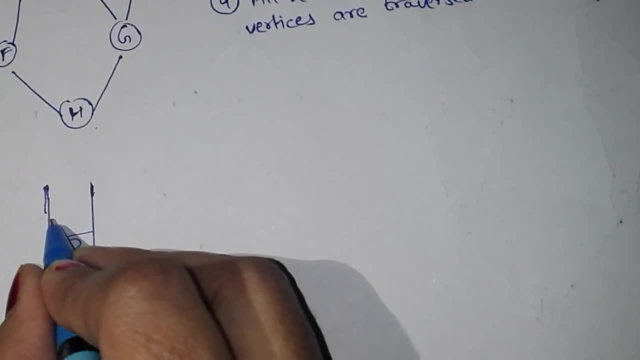 again connected with E. So here we write E, So our traversing is done. Now top element is G, So G is again connected with E. So here we write E, So our traversing is done. 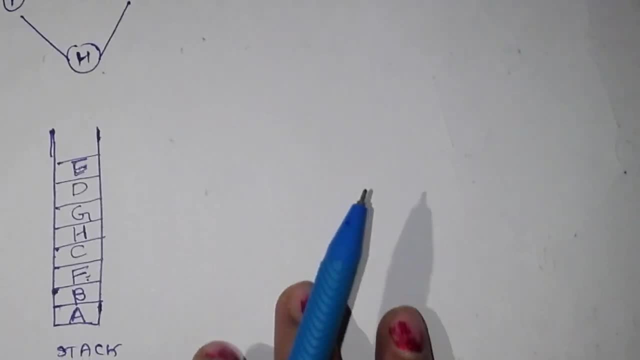 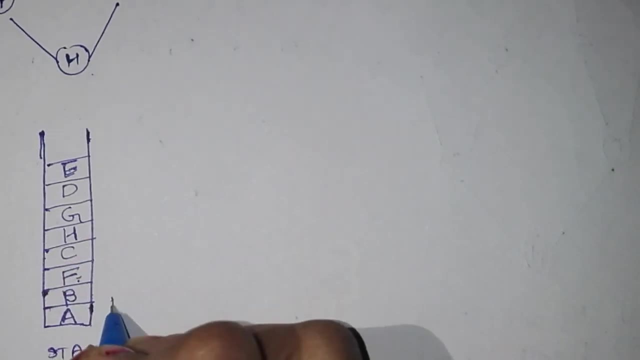 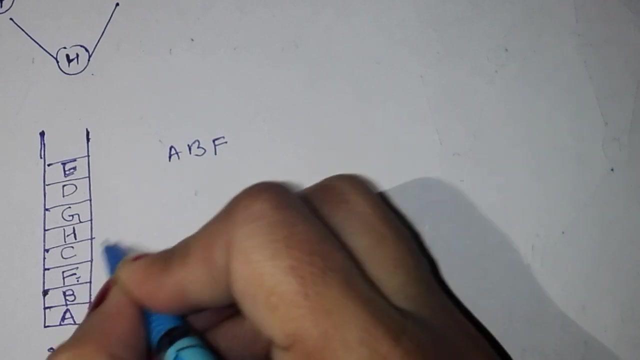 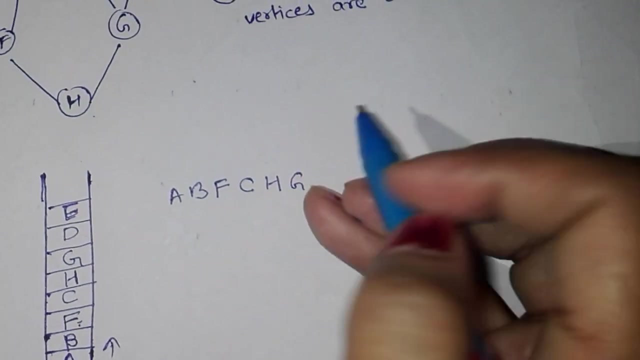 So our traversing is completed. We create a spanning tree with minimum number of edges. Here the traversing is A. in this way, First we traverse A, then B, then F, then C, then H, G, D and E. Okay, friend.